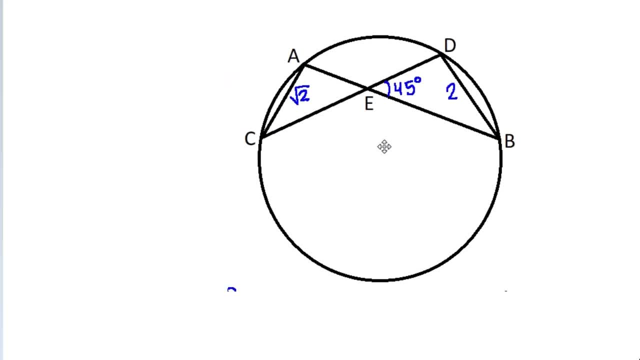 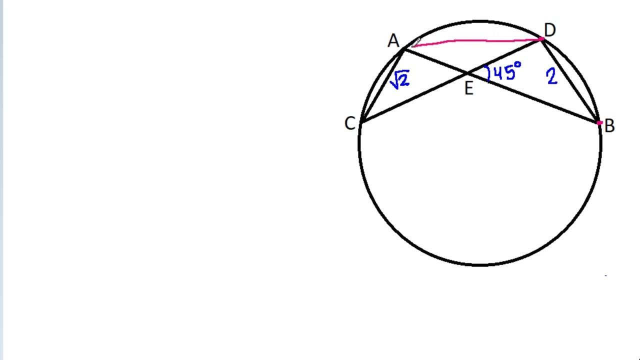 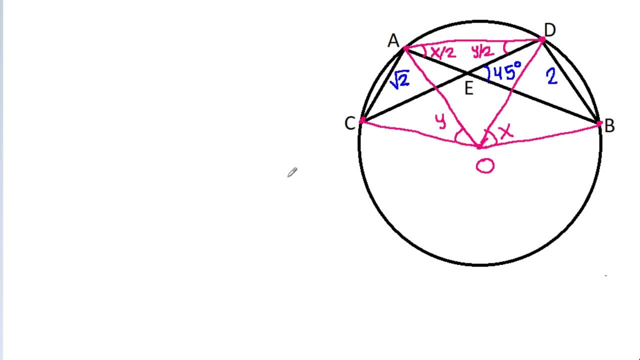 on the circle, then it will make an angle of y by 2 on the circle, then it will degree. And now inter angle, AED. it is AED. this angle is x by 2, this angle is y by 2, and this: 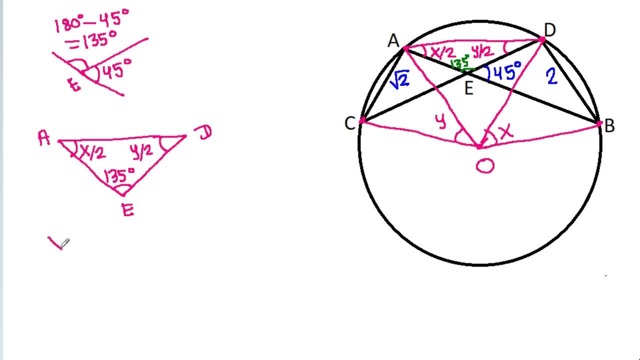 angle is 135 degree, So 1 pulls up, it will be equal to 180 degree. So it will be equal to 45 degree, So it will be 90 degree. That means y, it will be 90 degree minus x. 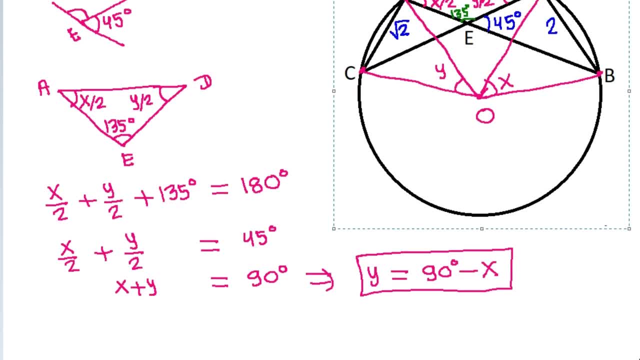 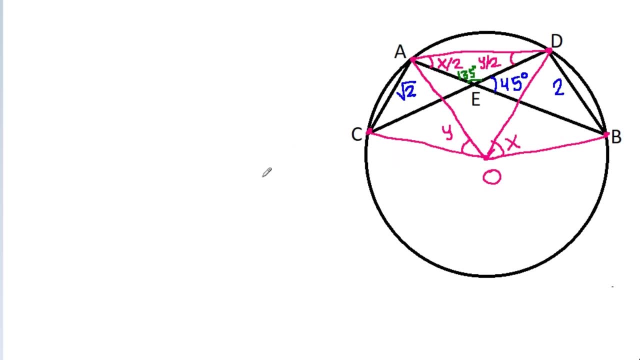 And now inter angle BOD here, BO, it will be equal to DO, it will be equal to AO, it will be equal to CO, that will be radius, Suppose R. so BO is R, DO is R, CO is R and AO is R. And now 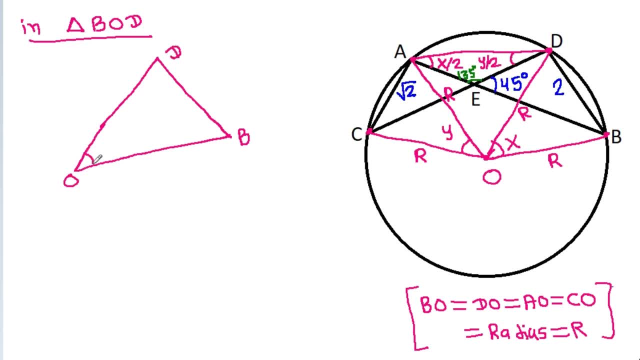 in BOD this angle is x, BO is R, DO is R and BD is 2.. So cos x, it will be equal to R square minus R square, minus 2 square by 2 times R times R, And cos x it is equal to 2 R square minus 4 by 2 R square. 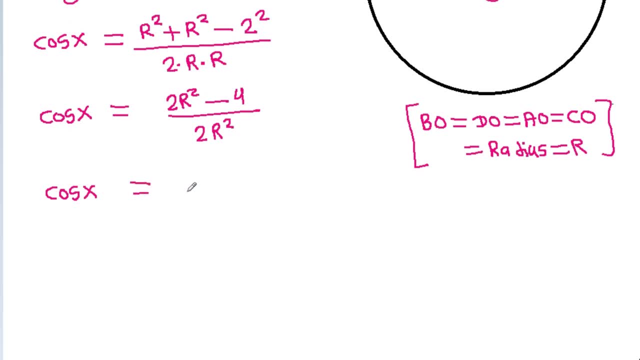 And cos x, it is equal to 2 R square by 2 R square, minus 4 by 2 R square, And 2 times 2 is 4.. So cos x, it is equal to 1 minus 2 by R square. 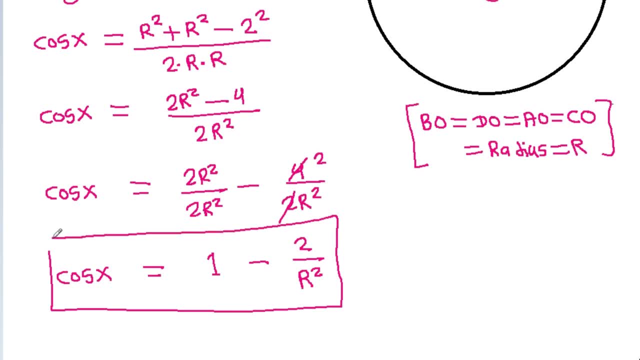 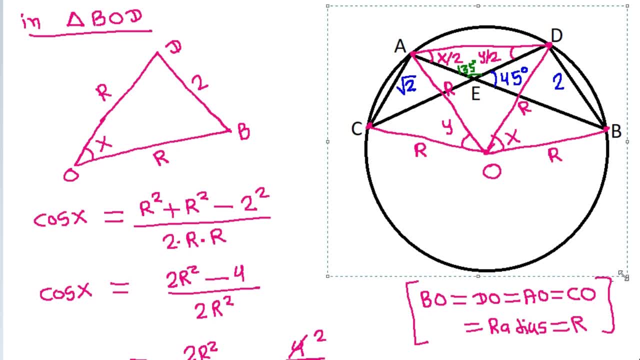 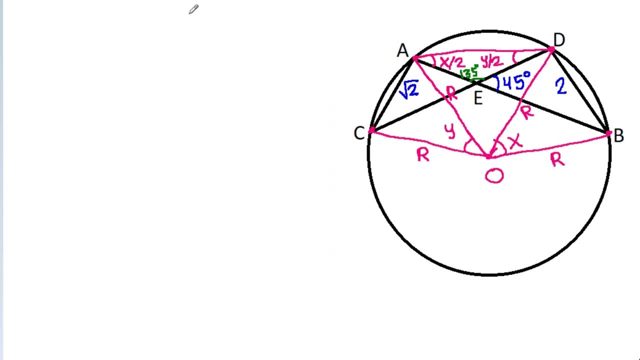 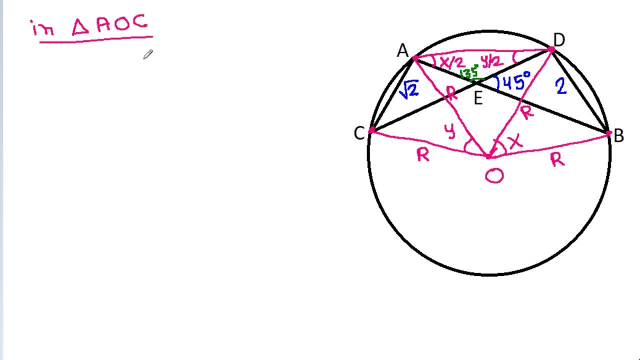 angle: AOC, it is AOC, AO is R, CO is R and AC is a square root of 2 and this angle is Y, So, COSY, it will be equal to R square plus R square minus A square root of 2, A. 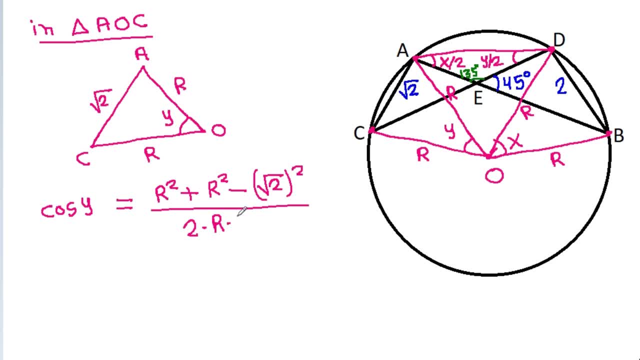 square by 2 times R times R, and it is COS and Y. it is 90 degree minus X, It is equal to 2R square. So it will be minus 2 by 2R square and COS, 90 degree minus theta, it is equal to sine. 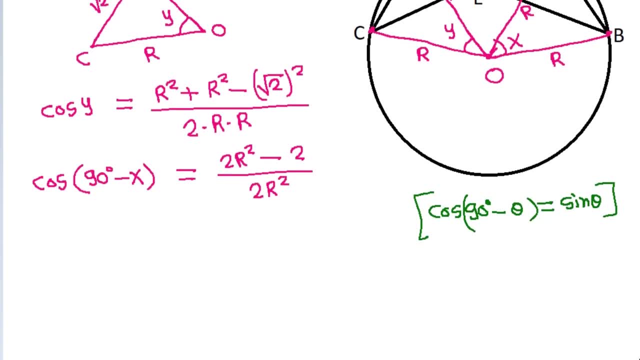 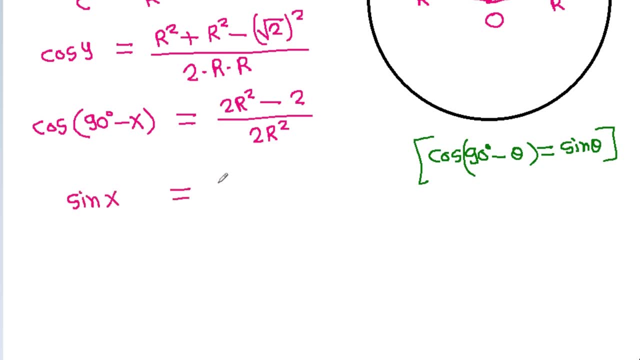 theta, So it will be: sine X is equal to 2R square by 2R square minus 2R square by 2R square minus 2 by 2R square. So sine X it is equal to 1 minus and 2 will get cancelled. so it is 1 by R square and. 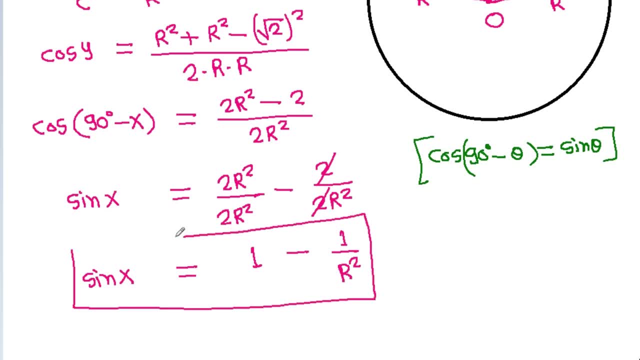 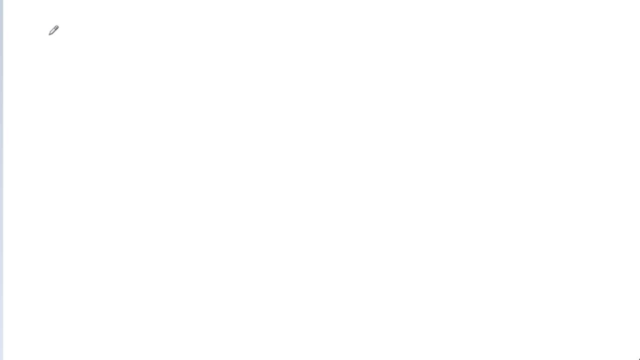 we know that MATTU X is equal to two by 2R square plus sine X is equal to two by 2às, four times plus sine X. So this is what it will be, And this is the real mode of acceleration. now find mind this. 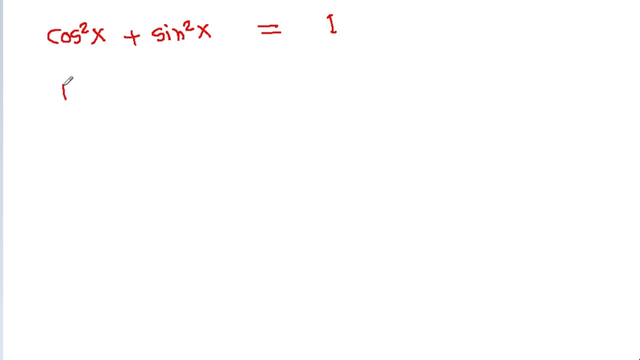 so the acceleration. so if this is equal to one, and we now simplify, so this is greater than or equal to zero. so this will be one. sin x, it is 1 minus 1 by r square, s square, it is equal to 1.. And now, if we take 1 by, 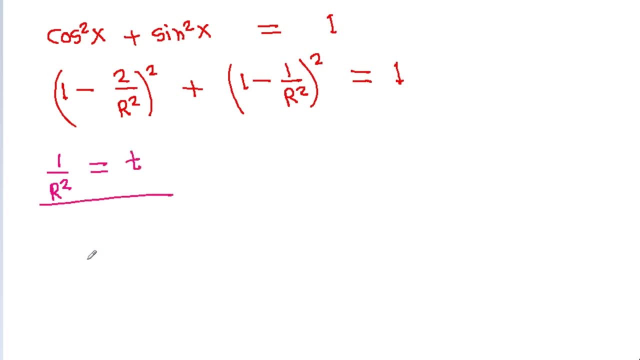 r square is equal to t, then it is 1 minus 2t s square plus 1 minus t s square is equal to 1.. And it is 1s square plus 2t s square minus 2 times 1 times 2t plus. and. 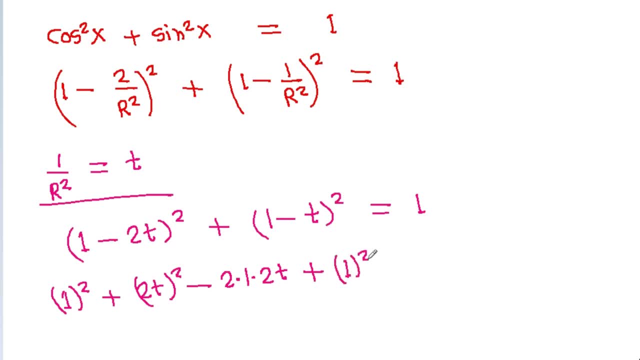 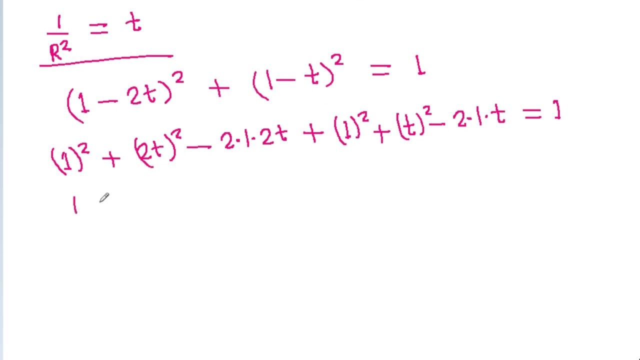 1 minus t s square, it will be 1s square plus t square minus 2 times 1 times t, that is equal to 1. And it is 1 plus 4t square minus 4t plus 1 plus t square minus 2t is. 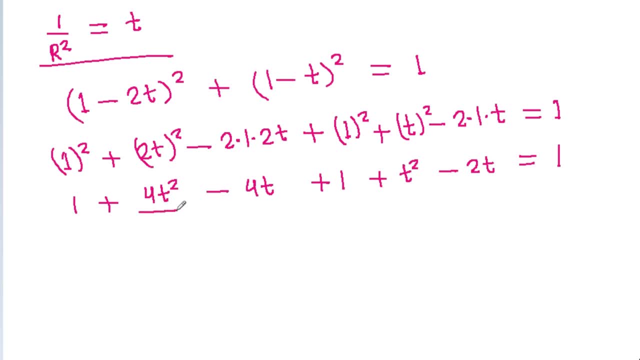 equal to 1.. And 4t square plus t square, it will be 5t square. And minus 4t minus 2t, it will be minus 6t. And 1 plus 1, minus 1,, it will be plus 1, that will be equal to 0. And it is. 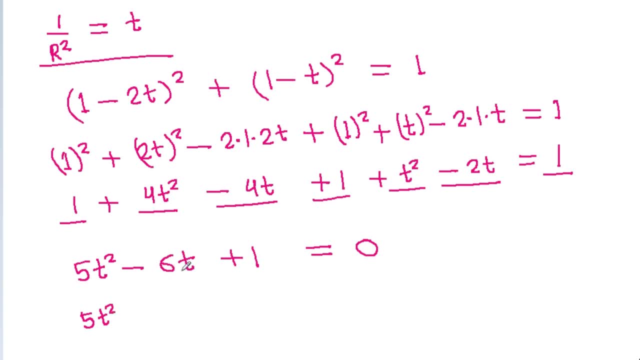 5t square minus 2t, that is equal to 1.. And it is 5t square minus 1, that will be minus 5t squared and minus 6t, it is minus 5t minus t plus 1, that is equal to 0.. And here we can. 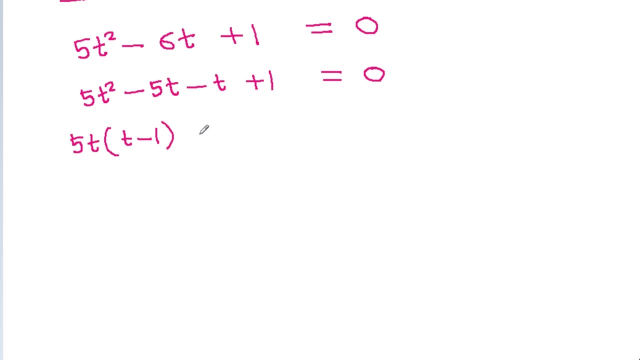 take 5t common and it is t minus 1 minus times t minus 1, that is equal to 0.. And now we can take t minus 1 common and it will be 5t minus 1, that is equal to 0. So either t minus 1, it will. 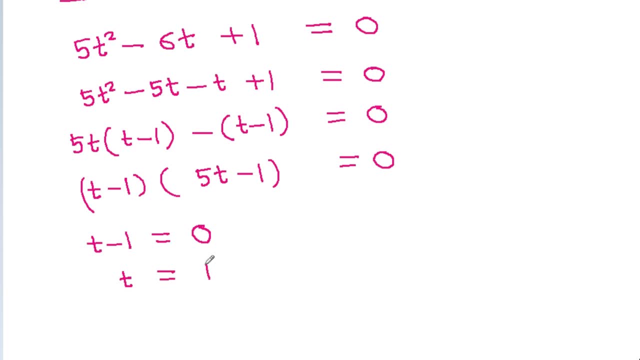 be equal to 0, that means t will be equal to 1.. And either 5t minus 1, it will be equal to 0, so t will be equal to 1 by t minus 1.. 5t and t is 1 by r square, that is 1. And r square it will be equal to 1.. So r it will. 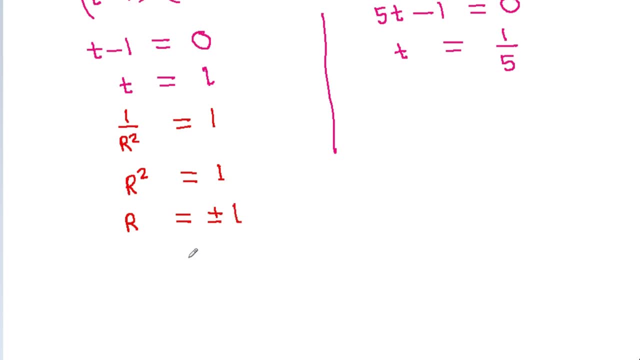 be equal to minus minus 1.. And r it is radius, that is length, so it should be positive. so r will be equal to 1, and here p is 1 by r square, that is 1 by 5,. so r square it will be equal to 5, and r it will be equal.